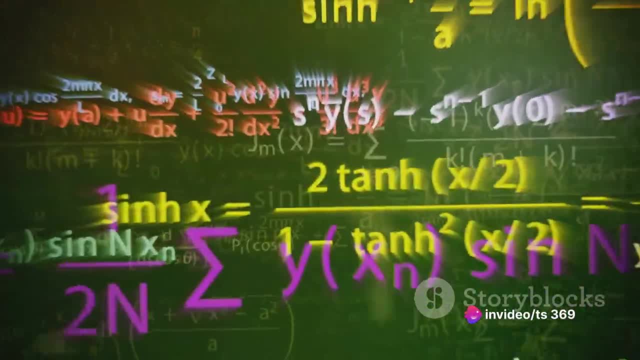 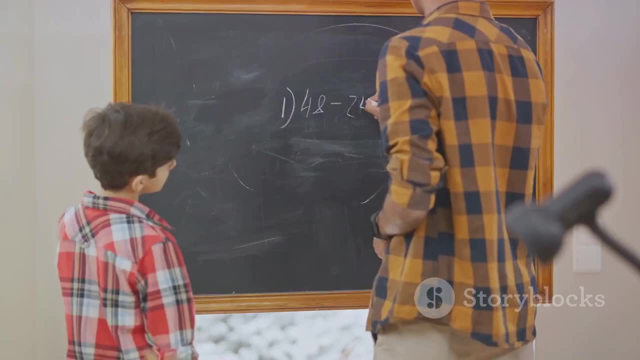 commerce, technology and even basic problem-solving all hinge on the principles of this subject. Let's break it down a little. Mathematics is a field of study that involves the properties and relationships of numbers, shapes and patterns. It's not just about crunching numbers or solving. 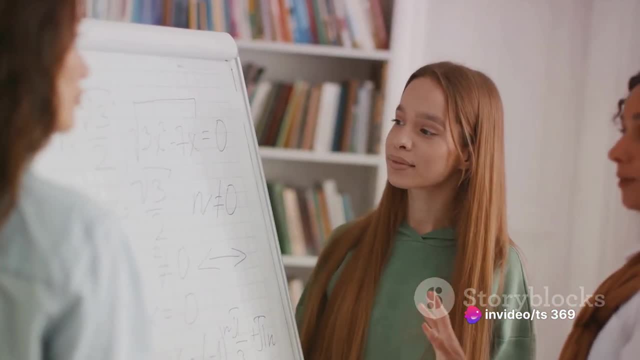 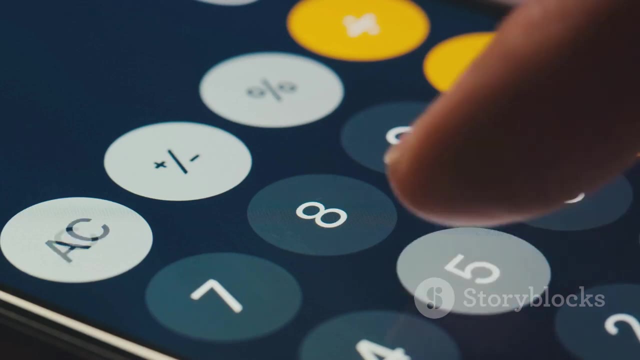 equations, but about understanding the logic and reasoning behind these processes. It's a system of thought and understanding that allows us to quantify, measure and describe our world in precise ways. Think about it: From the moment we wake up, we're immersed in maths. The time on. 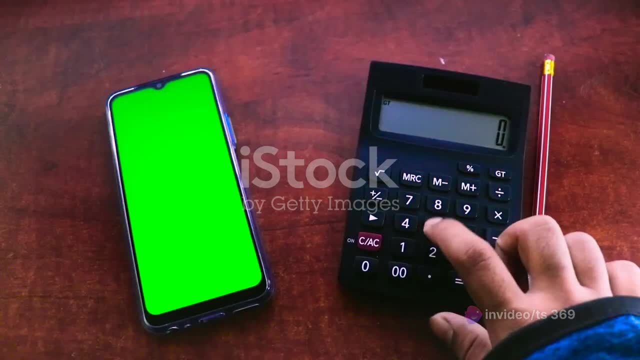 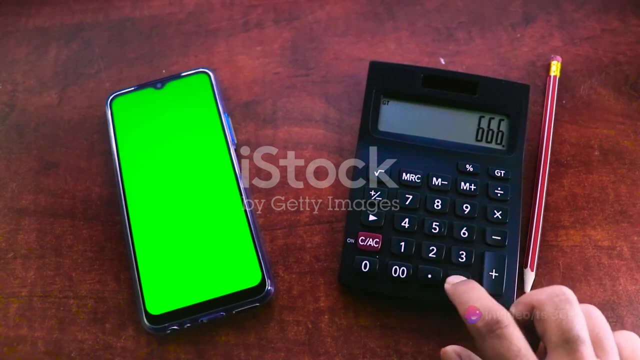 your alarm clock That's based on the mathematical concept of measuring time, The time in which you take to work or school. That includes understanding distance, speed and time- all mathematical concepts, Even the digital devices we can't seem to live without. 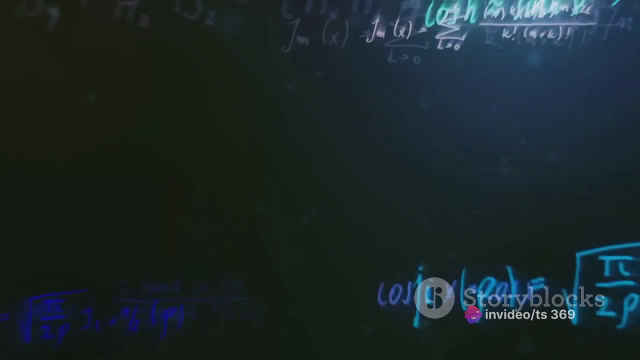 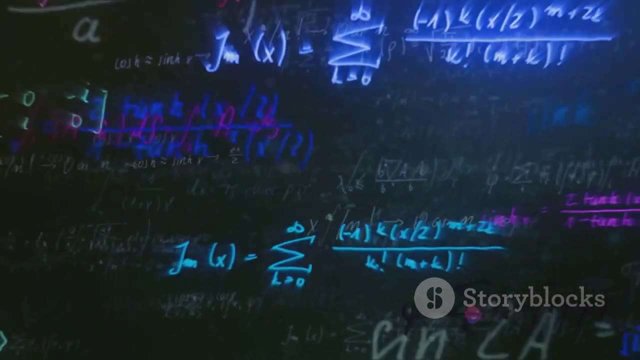 they operate based on complex mathematical algorithms. And it doesn't stop there. Mathematics is deeply embedded in various fields of study. In physics, it helps us understand the laws that govern the universe. In computer science, it forms the backbone of coding and programming. 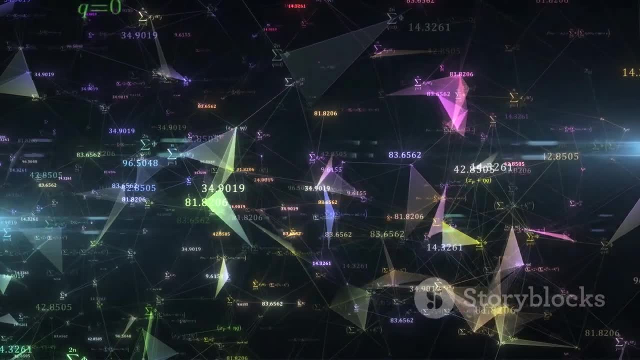 In economics, it provides tools to analyze and predict market trends. And in economics, it provides tools to analyze and predict market trends. And in economics, it provides tools to analyze and predict market trends. And in art and music it brings structure and balance. but don't let the complexity of maths intimidate you. 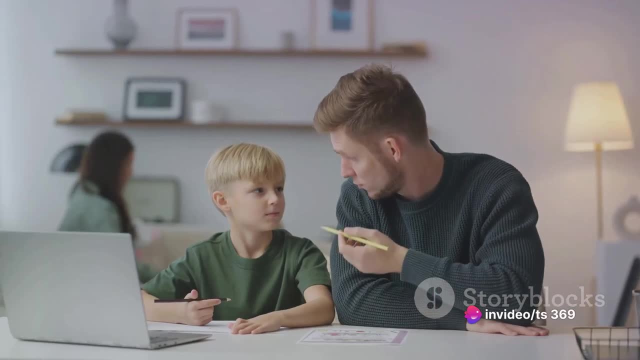 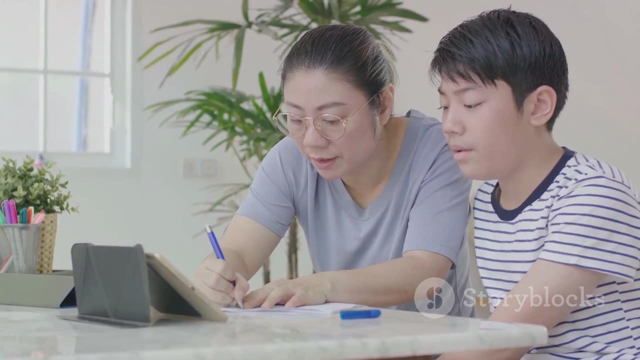 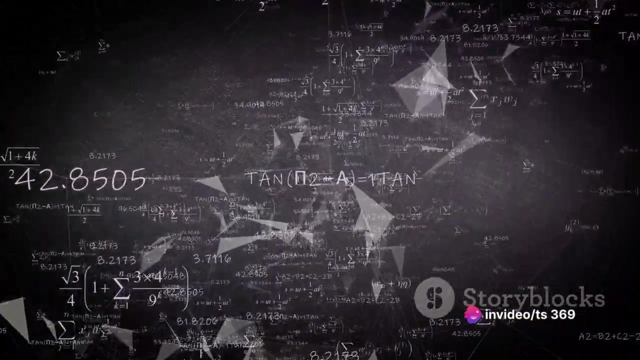 it starts from simple principles. basic arithmetic, like addition, subtraction, multiplication and division, are the building blocks of more complex mathematical ideas, and these fundamentals are something we all learn and use in our daily lives. so we see that maths is not just about numbers, but a tool for understanding and interpreting the world around us. it's not an isolated subject, but 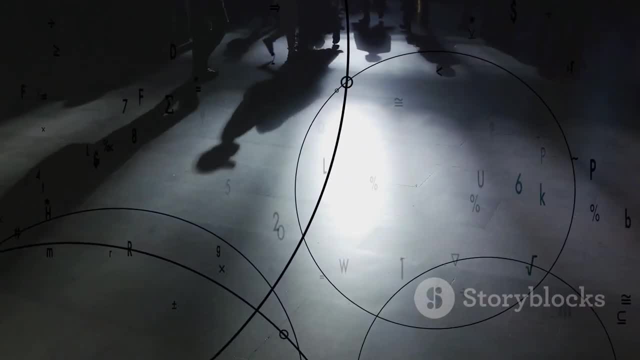 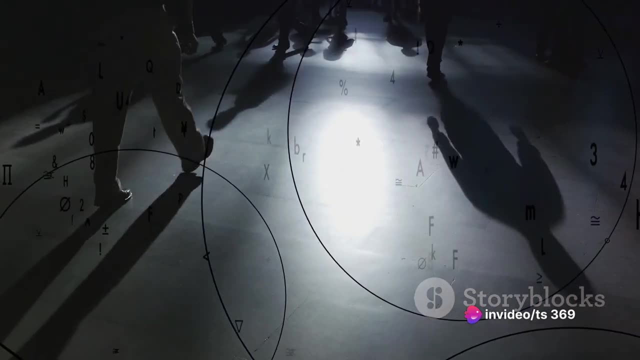 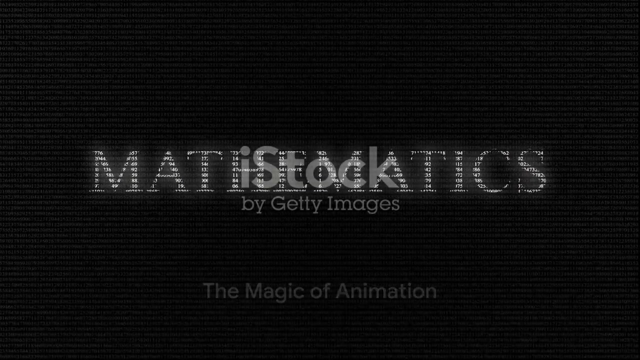 an integral part of life, woven into the fabric of our everyday experiences. so next time you come across a mathematical problem, don't shy away. embrace it as another opportunity to unravel the fascinating world of maths. now let's move on to the world of animation, a realm where creativity 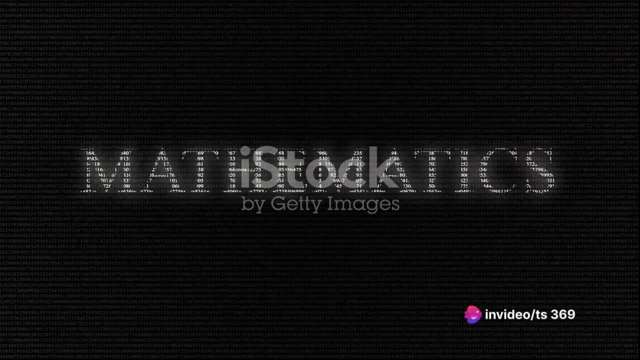 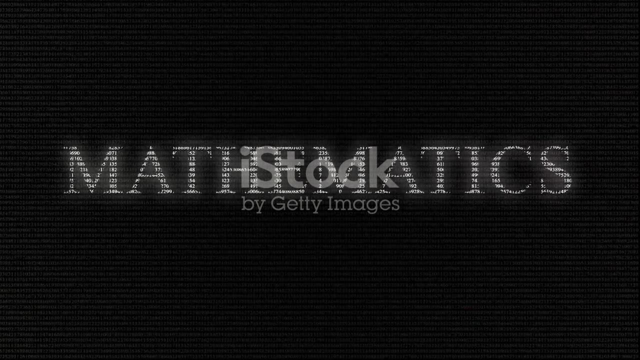 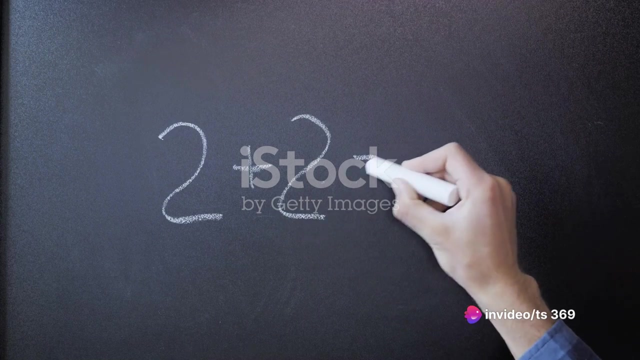 meets technology. animation, in its essence, is the art of bringing static images to life, creating the illusion of movement through a rapid sequence of pictures. it is where imagination takes flight, soaring beyond the limits of reality, and the world of animation is the world of animation beyond the confines of reality. animation is not just about cartoons or movie special effects. 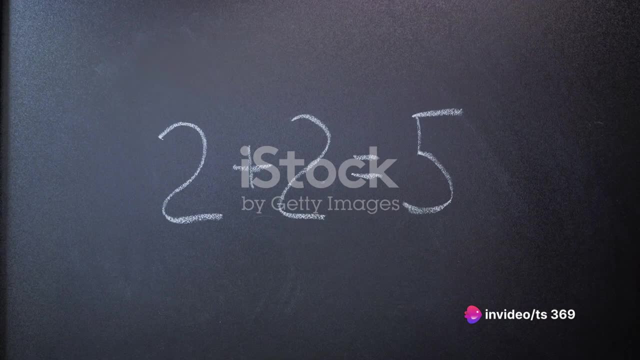 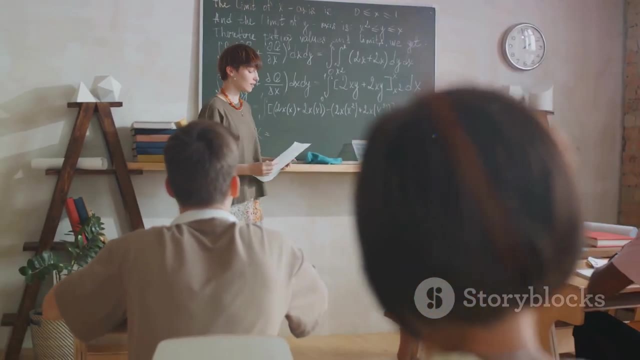 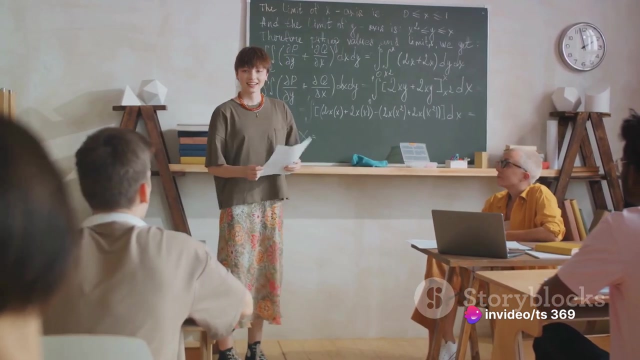 it's a powerful communication tool used across a myriad of industries, from advertising and gaming to education and scientific visualization. there are several types of animation, each with its unique allure. traditional animation, often reminiscent of classic disney films, involves meticulously hand drawing each frame. stop motion animation breathes life into inanimate objects. 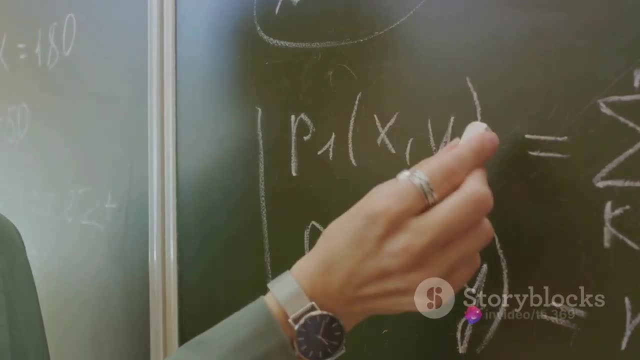 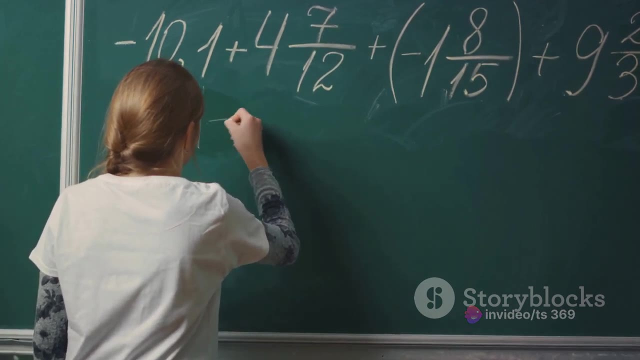 frame by frame in a labor-intensive way. animation is not just about cartoons or movies: special effects in a labor of love. computer animation, on the other hand, uses digital models and software to create both 2d and 3d animations. it's this type that has revolutionized the animation industry. 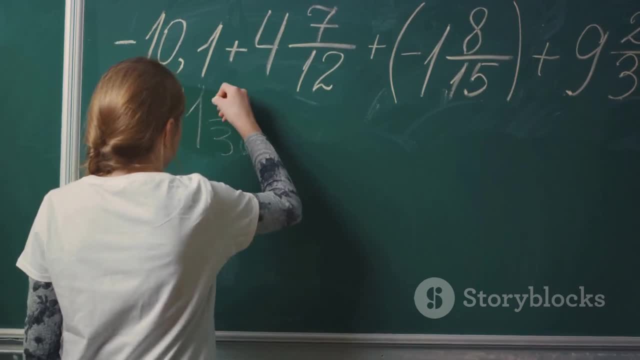 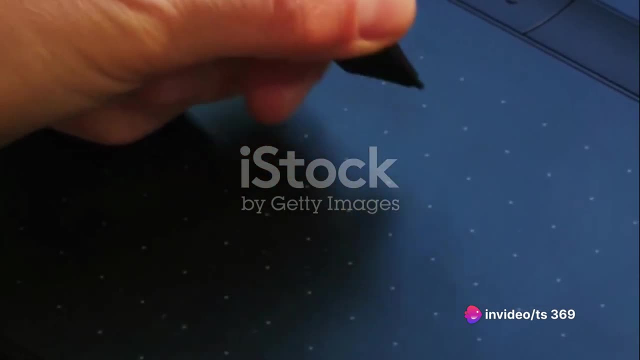 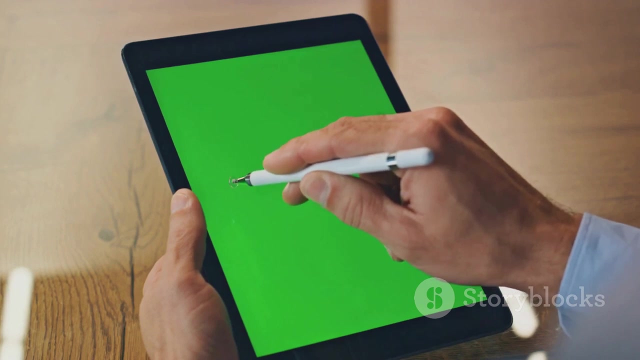 bringing us the hyper-realistic animations we see in modern films and video games. the process of creating animation is a complex dance between art and technology. it begins with a concept or story, which is then visualized through storyboarding. the characters and scenery are designed and then brought to life through animation. 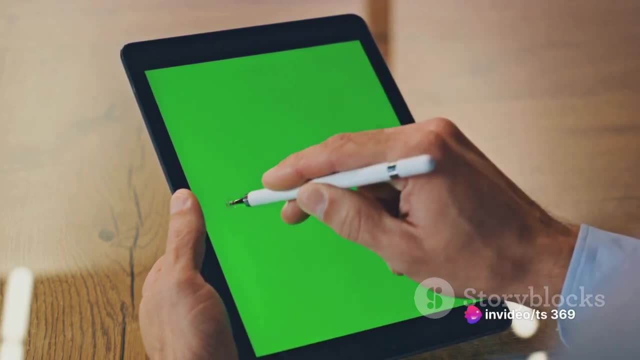 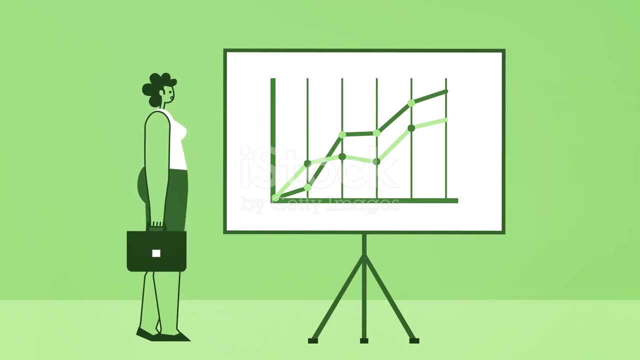 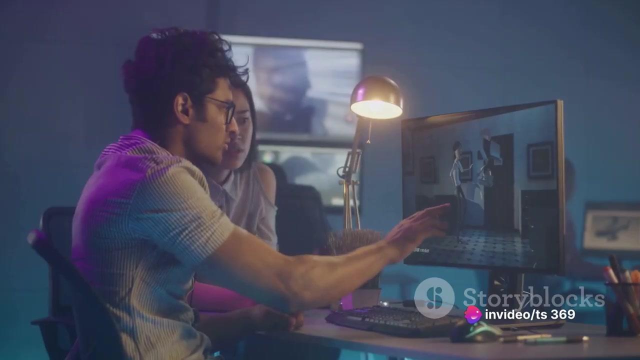 it's a process that requires a blend of creativity, technical skills and an eye for detail. the skills required in animation are as diverse as the types of animation itself. an animator needs a strong grasp of anatomy, motion and art to create believable characters and movements. they also need to master various software and technologies, but perhaps the most important skill is storytelling. 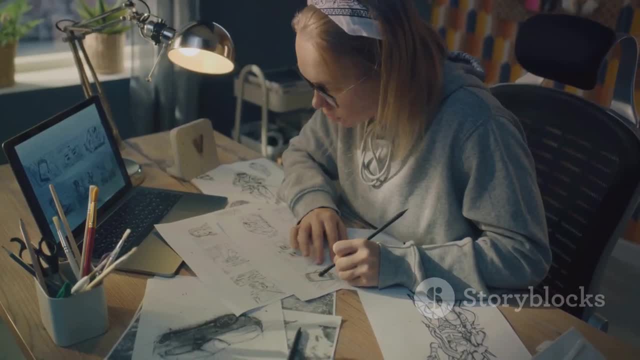 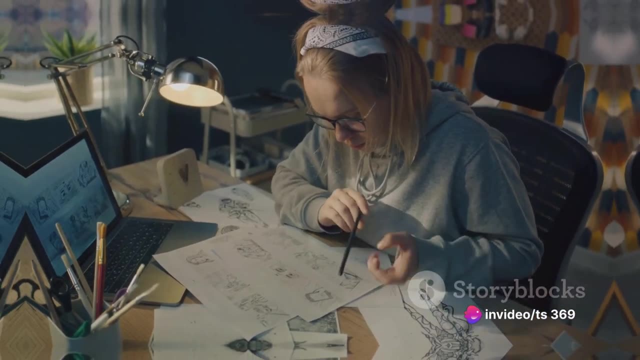 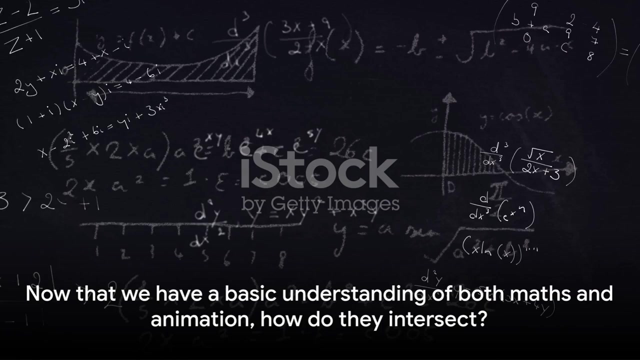 after all, the aim of animation is to tell a story that captivates, entertains or educates the audience. as we can see, animation is a dynamic field that brings stories to life. now that we have a basic understanding of both maths and animation, how do they intersect? let's dive right in. 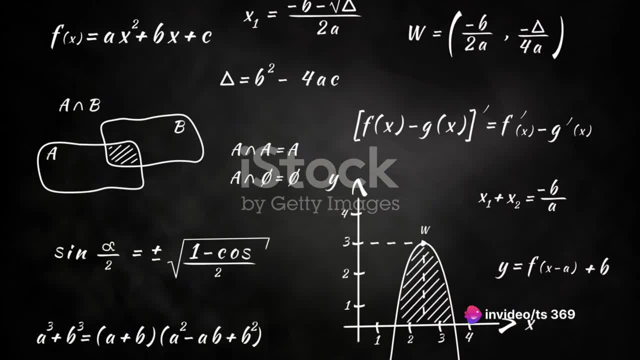 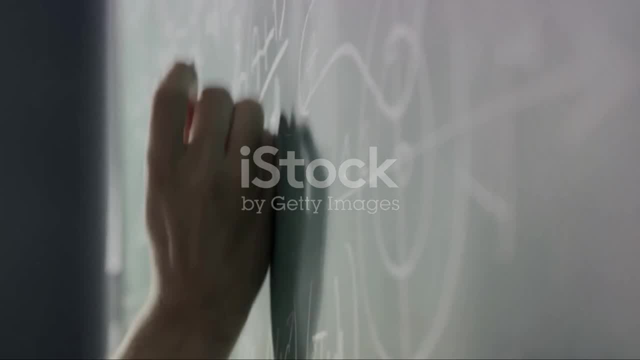 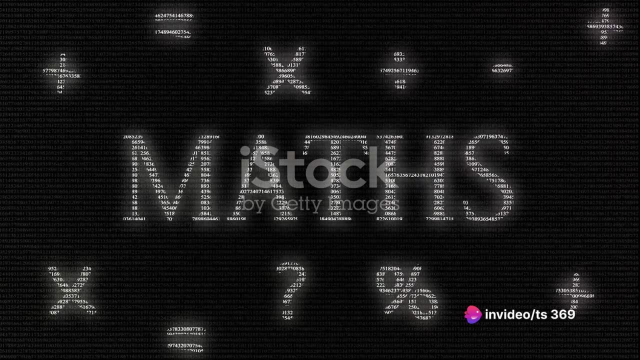 at first glance, mathematics and animation might seem like strange bedfellows, yet they share a profound connection. mathematical principles are the backbone of creating realistic movements and effects in animation. take, for instance, the concept of geometry. geometry helps animators create shapes that are integral to the animation process. It's the line segments, the polygons, the curves and 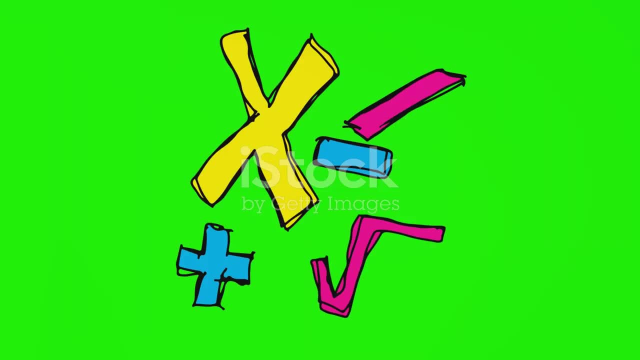 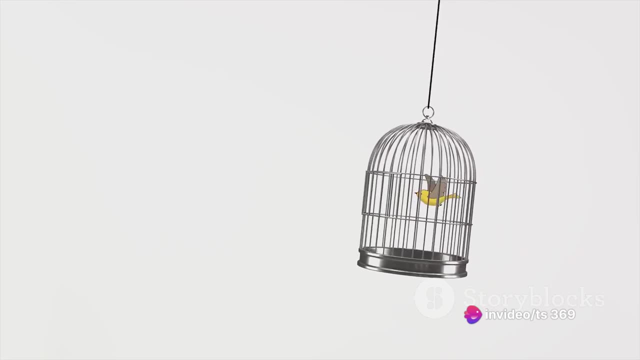 the angles that breathe life into a character or an object. It is geometry that gives a bumblebee its rounded shape or a skyscraper its sharp edges in an animated world. Now let's talk about trigonometry, a branch of maths that deals with the relationships between the sides and angles. 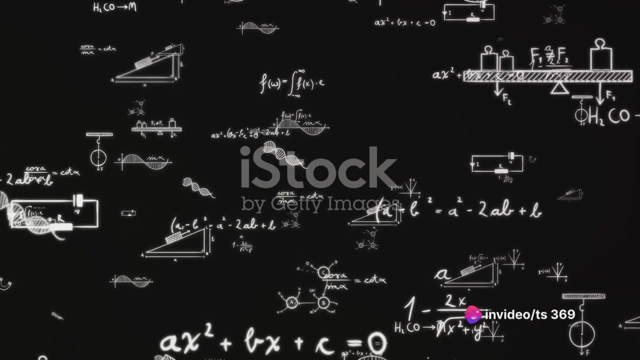 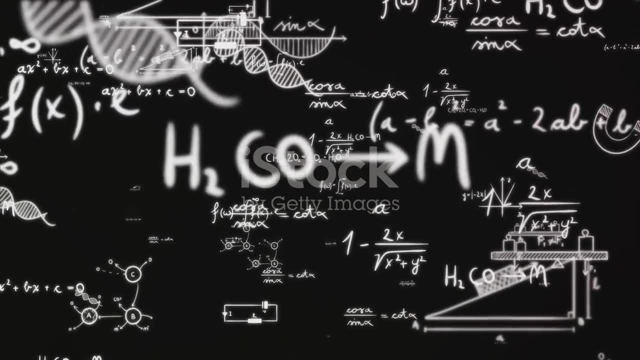 of triangles. This might sound unrelated to animation, but it's actually crucial in creating movement. Imagine a character swinging a baseball bat or a bird flapping its wings. Trigonometry helps in calculating the arc of these movements, making them look natural and fluid. 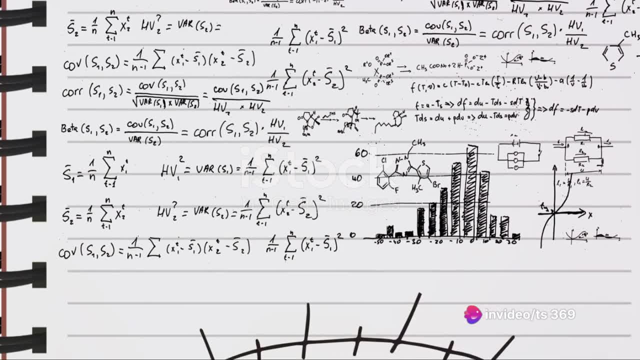 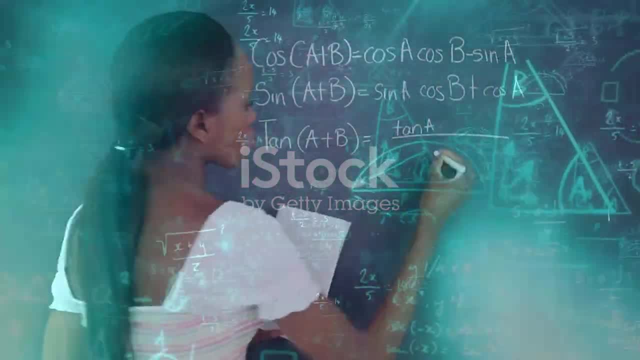 Another mathematical principle that plays a big role in animation is calculus. Calculus helps animators understand how things change and move. For instance, when an animated character jumps off a cliff, calculus helps determine the trajectory of the jump, the speed of the fall. 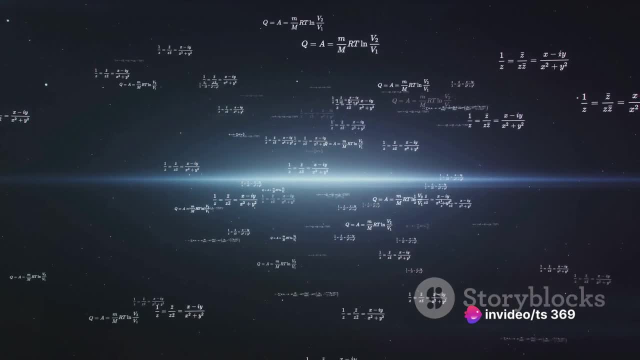 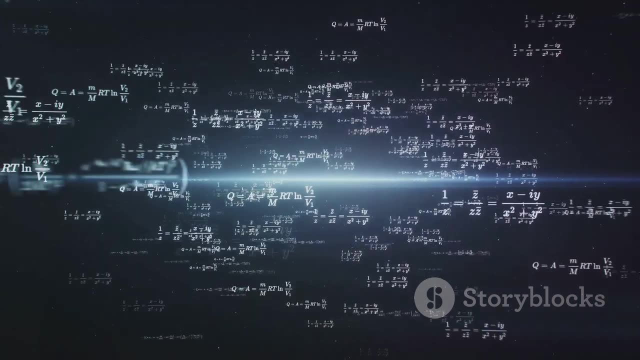 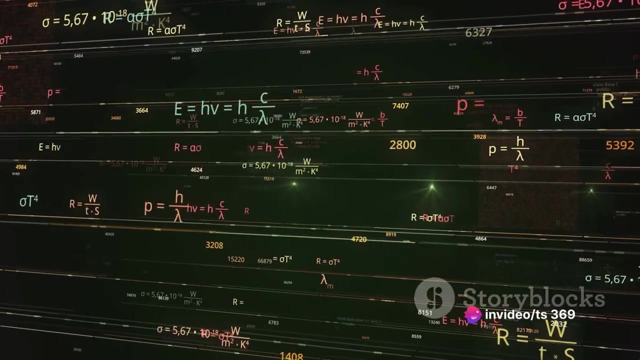 and the impact of the landing. Finally, let's not forget about physics. While not strictly mathematics, physics is deeply rooted in mathematical principles. Physics is what makes the world of animation believable, providing gravity, friction and inertia. It's what makes a character's hair flutter in the wind or a car skid around a corner. 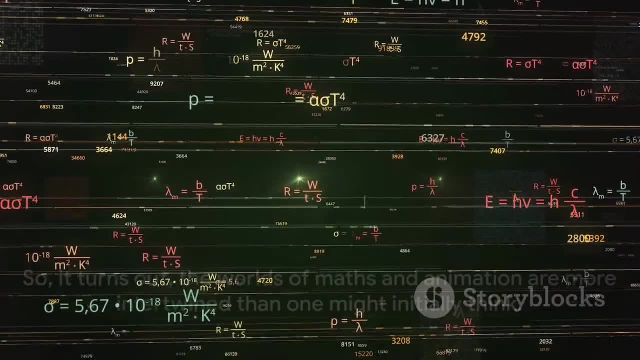 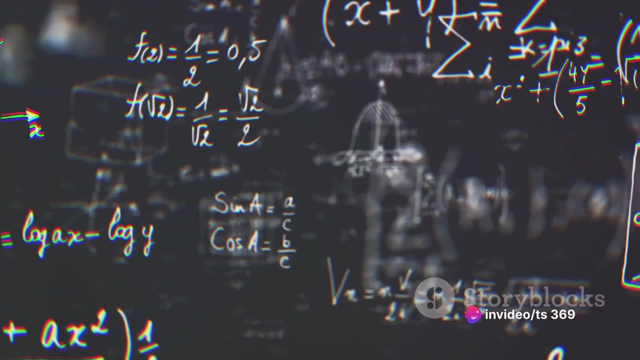 So it turns out, the worlds of maths and animation are more intertwined than one might initially think. In our journey today, we've explored the relationship between maths and animation, we've navigated through the dynamic world of numbers and we've explored the dynamic world of numbers and we've explored the dynamic world of numbers. 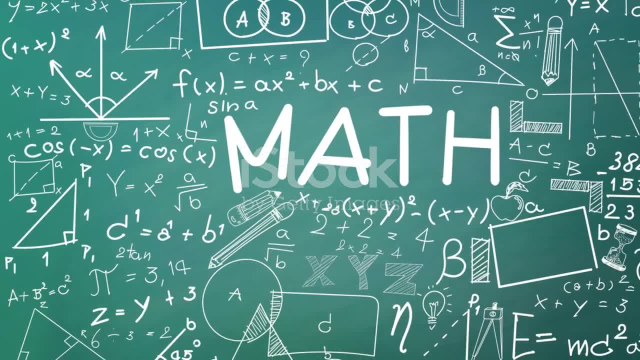 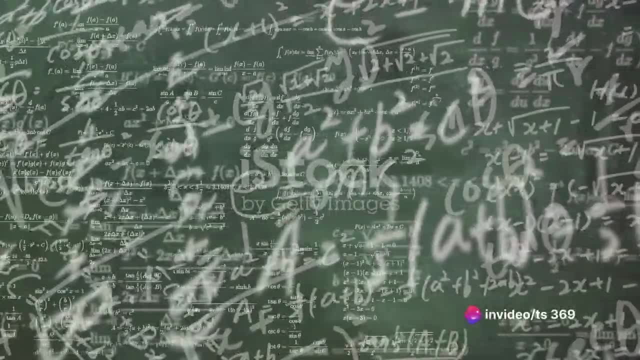 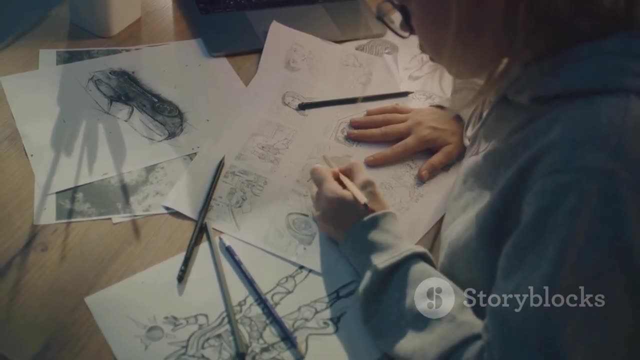 and variables, discovering how they form the backbone of the animations we so dearly love. From the simplest of cartoons to the most complex of CGI masterpieces, we've seen how mathematics plays an integral role. We dived into the realm of animation, witnessing the magic that brings our 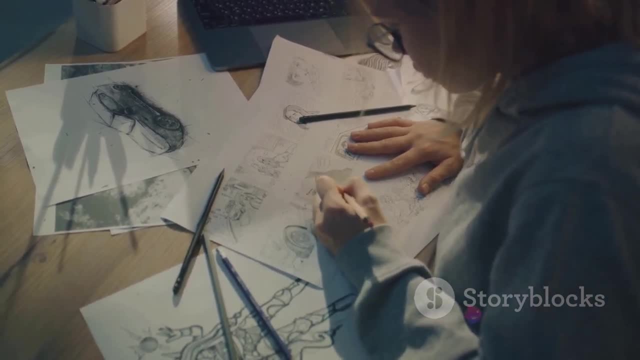 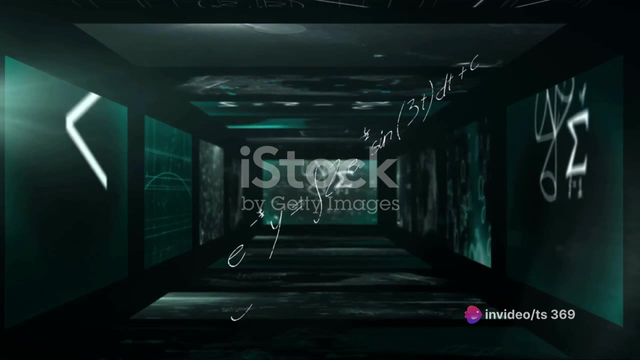 favorite characters and stories to life. We've seen how animation in its various forms has the power to evoke emotions, tell compelling stories and create unforgettable experiences. Then we witnessed the enchanting dance between maths and animation. We saw how the precision and logic of maths meld. 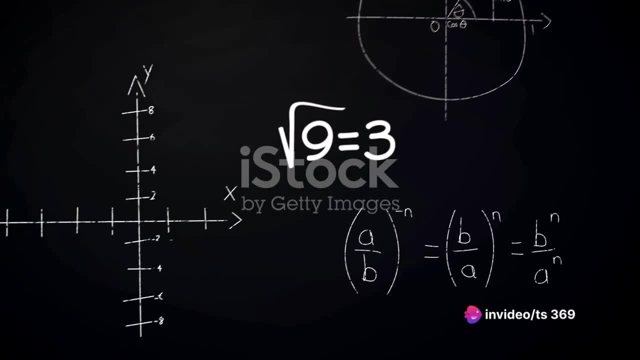 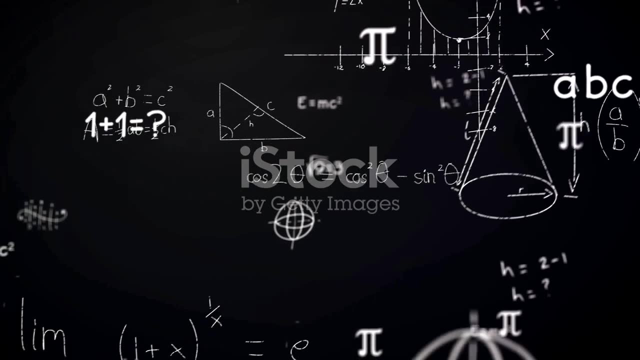 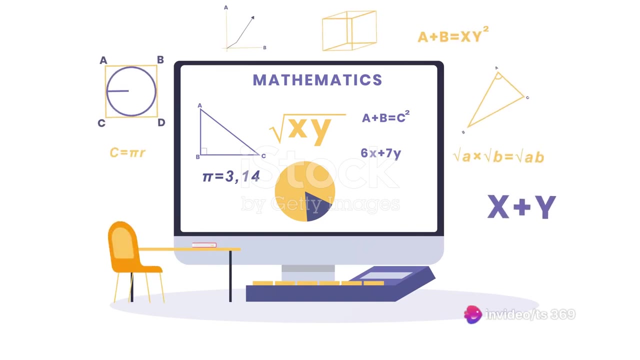 with the creativity and imagination of animation to create spectacular visuals. We've learned that the intricate movements of animated characters, the surreal landscapes and the mesmerizing special effects are all dictated by mathematical principles. We've also emphasized the importance of both maths and animation in various fields, For 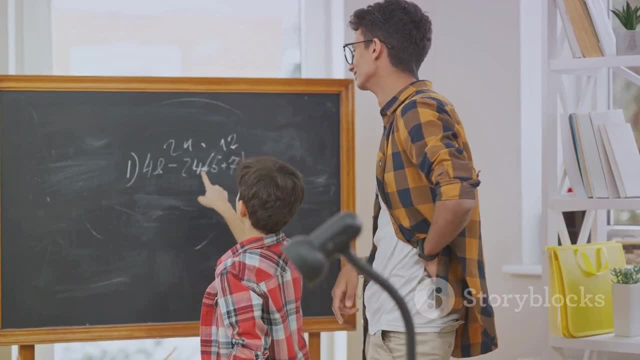 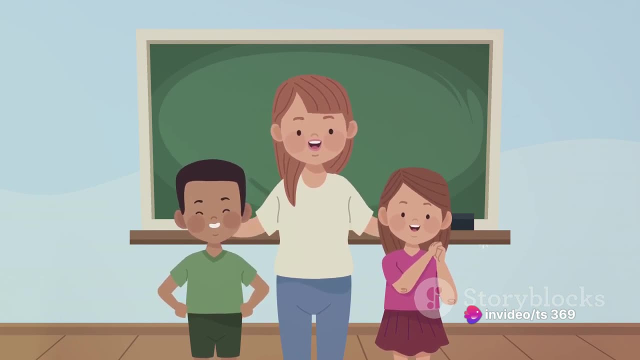 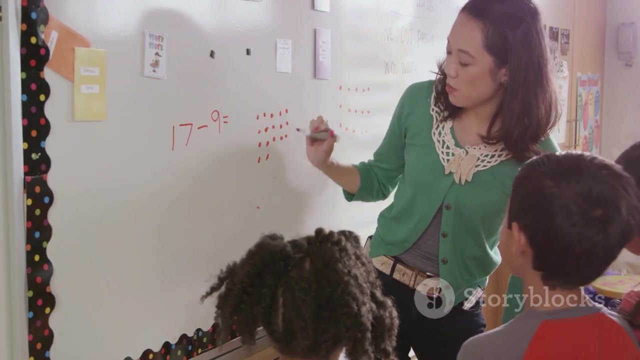 instance in the gaming industry. the combination of maths and animation is essential to create realistic environments and character movements In education. animation makes complex mathematical concepts more accessible and engaging for students. As we wrap up, let's not forget the intriguing intersection of these two worlds. The harmony between maths and animation is